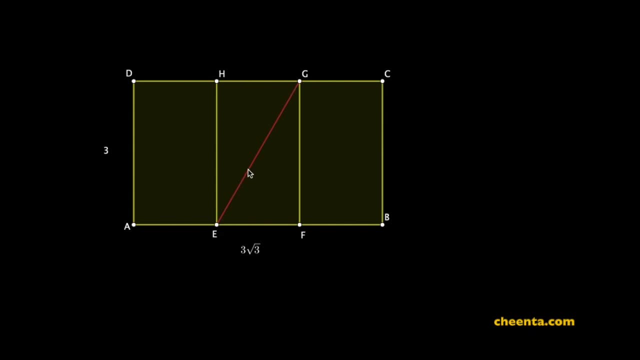 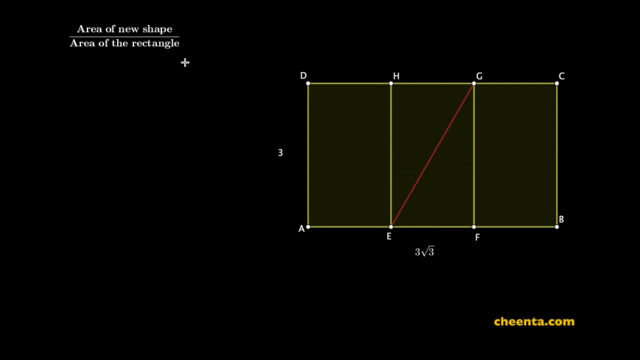 paper. We will be folding this portion of the paper across this red line and we want to find out the area of the new shape, that is, the one that we get after folding, and the ratio of that with the ratio area of the actual rectangle. So a variety of ways of 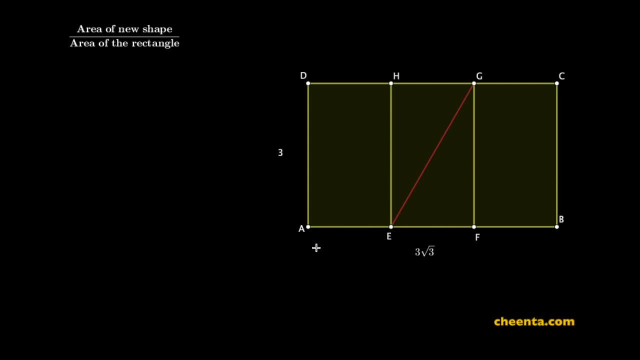 doing this, and you can find beautiful solutions online. We are, however, more interested to visually fold the paper using the software's power, and see what's going on. So this is the portion this EGCB, This is the portion that we want to fold, and we want to fold it across EG. So toward that end, let's start. 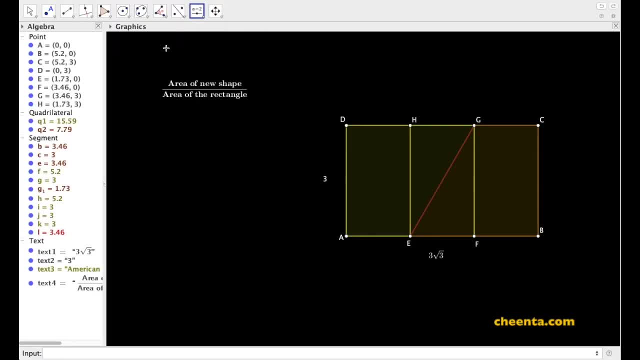 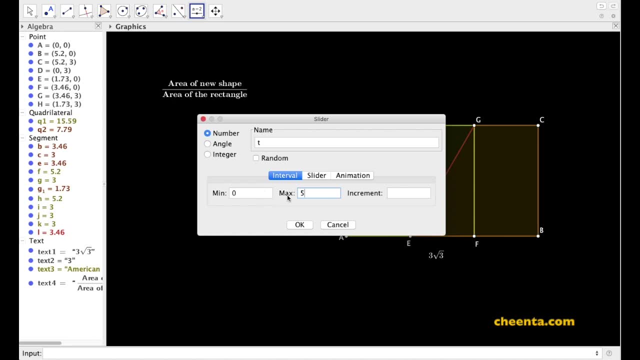 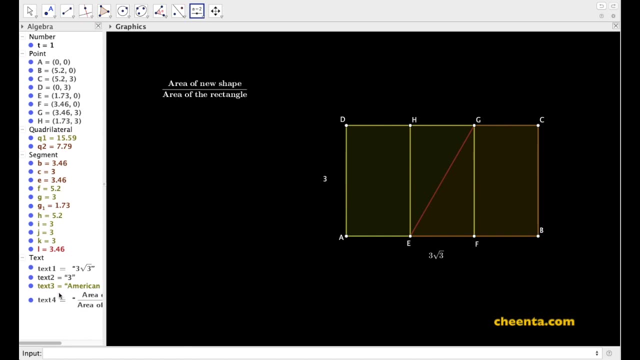 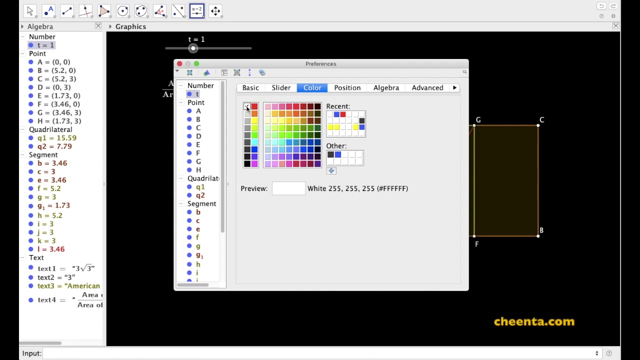 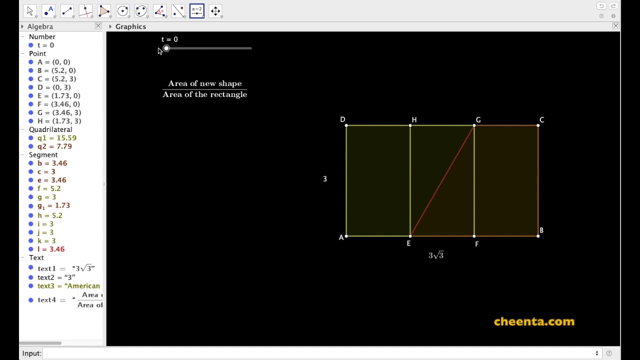 with the slider. That will give us the angle- Let's call it T- from zero to high, and let's put this slider in white color, maybe, So we can. we can now change the slider. It will work as a variable. So I initiated a T. 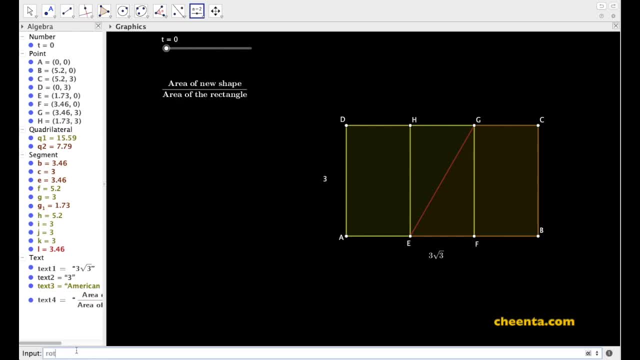 equal to zero. and now we want to rotate this object. which object is Q2? object Q2 is this red portion of the paper, So let's call it Q2 by angle T. T is initiated at zero, but it can go up to 180. 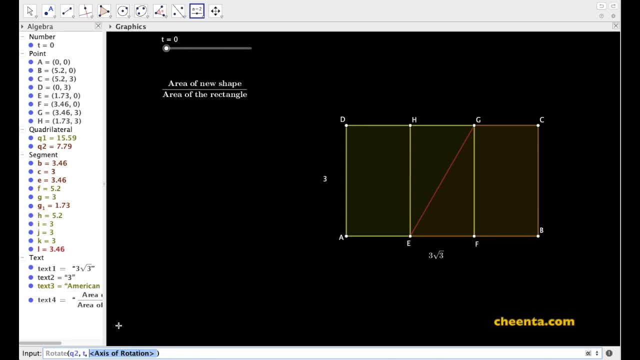 degrees and the axis of rotation needs to be EG. Now the name of the segment is E in this particular case. Okay, so we have the rotation defined, which is Q2 prime, and if we change this to from zero, if we go on up to 3.14, we see that nothing is happening. The reason: 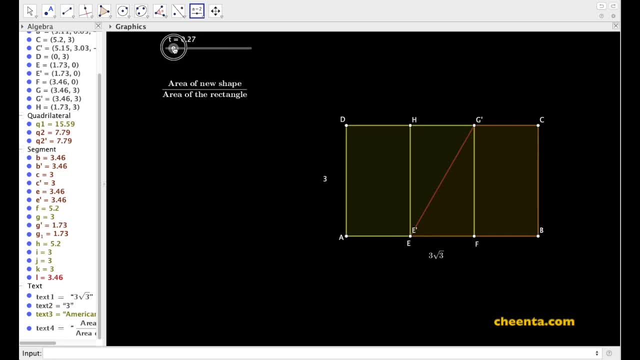 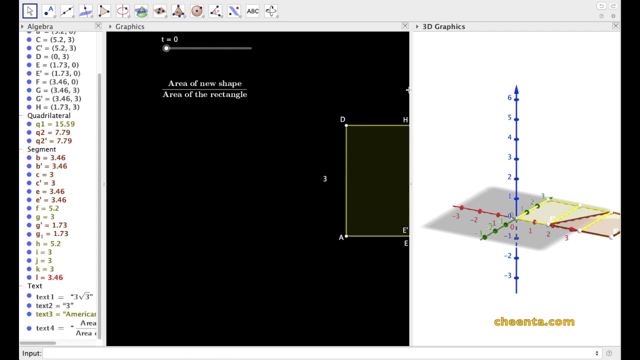 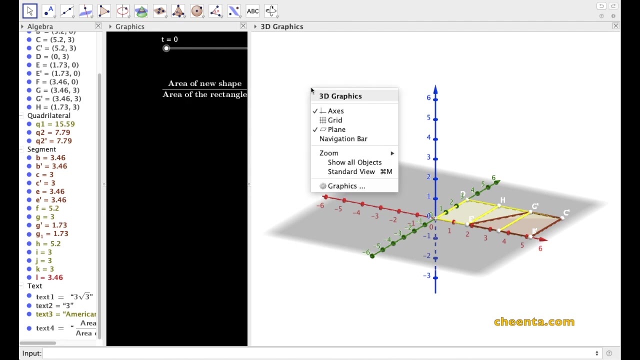 is that we are in two-dimensional world and suddenly in two-dimensional world. two-dimensional world, we cannot really revolve around a segment, so let's go to the three-dimensional world. let's go to three-dimensional world, initiate some 3d graphics here and to make it more attractive, what I'll do is: I'll change. 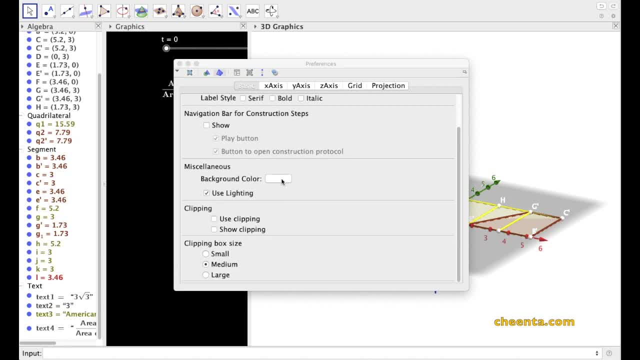 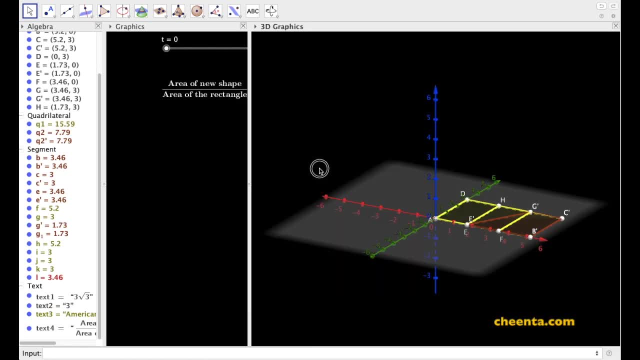 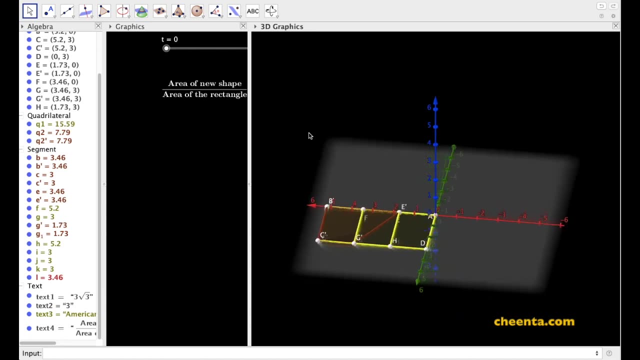 the graphics, color to background, color to black, make it a little bit more visually fun, and we really don't need the axis, though we can have some fun with it, but we don't need the axis, so let me get rid of the axis anyway, and we have this. 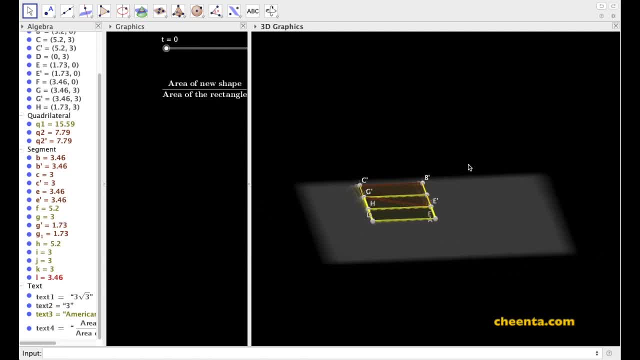 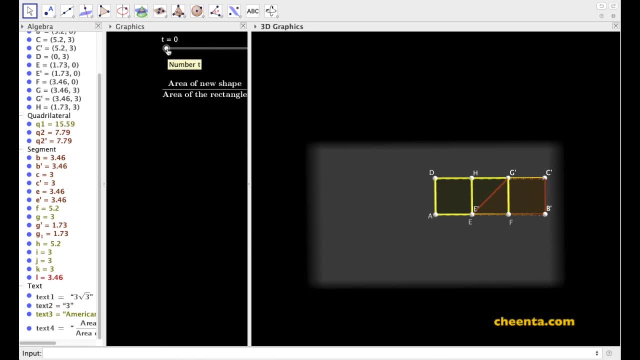 beautiful looking rectangle with a portion of it that we want to fold. okay, now, let's now use the slider. you see that what's happening is this rectangle is folding, and if I go all the way, if I go all the way to three point one, four, that's, that's pi, that's approximately pi. we get the rotated figure. so 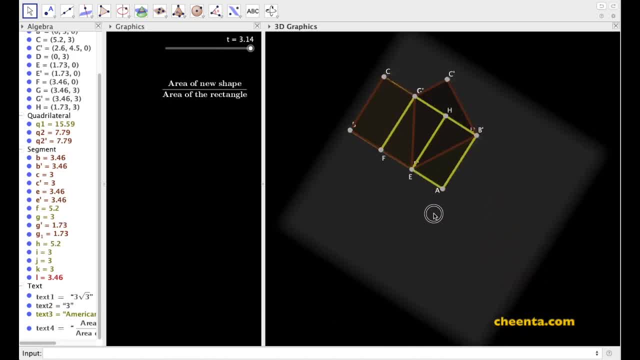 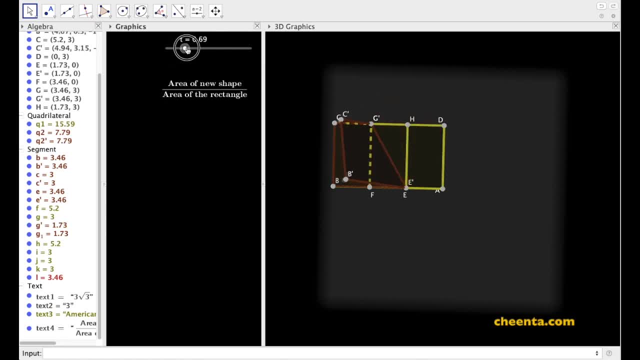 if you don't look at this from beneath the figure, you get a better idea. so this is the paper and it gets folded into this position. it's kind of fun because after folding you get this portion of the shape and this, this particular part, gets chopped off. obviously it got folded here and now. 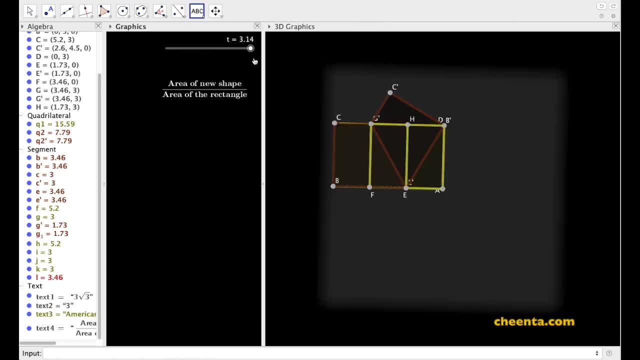 and now you can actually use a little bit of a little bit of intuition to see that this particular triangle that I marked with one initial rectangle had six of these triangles. so one, two, three, four, and if you chop this off into two parts you'll get six. so maybe I can just join this segment and let's change the.